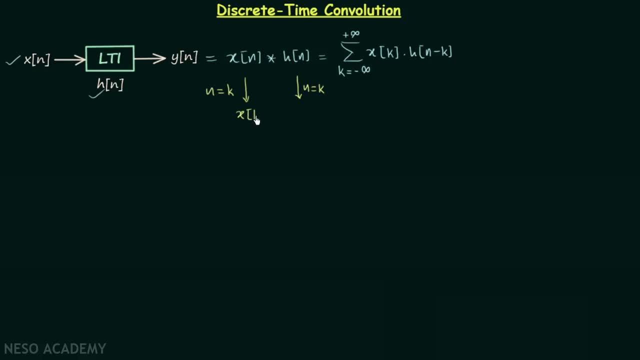 And after this we will have signal Xk in place of signal Xn and we will have signal Hk in place of signal Hn. Now we will leave alone signal Xn, xk and we will focus on signal hk. Let's perform time reversal operation on. 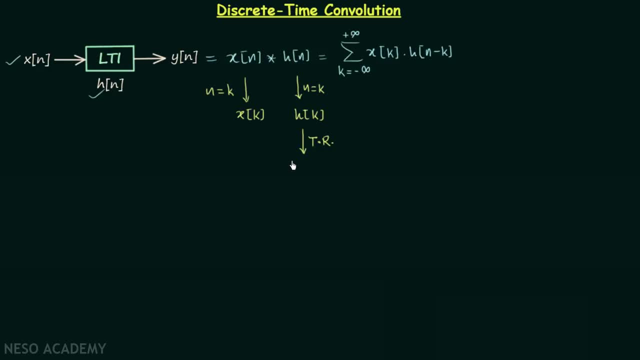 signal hk. After performing the time reversal operation, we will have a new signal that is h minus k, and once we have this signal, we will perform another operation, which is time shifting operation, and we will perform the time shifting operation by n. This will give us a new signal: h minus k plus n. We can. 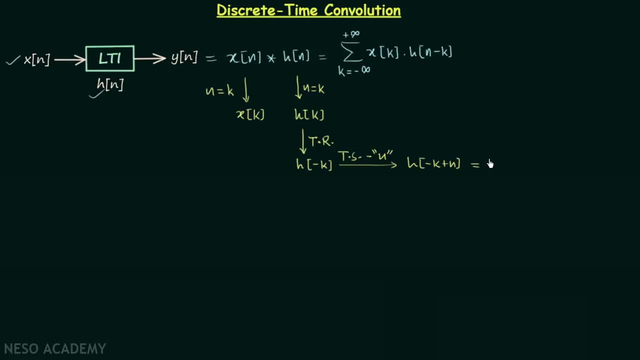 write h minus k plus n, equal to h n minus k. Now look at this result. We are having xk multiplied to h n minus k. You can see that we have xk here and we have obtained h n minus k after performing the time. 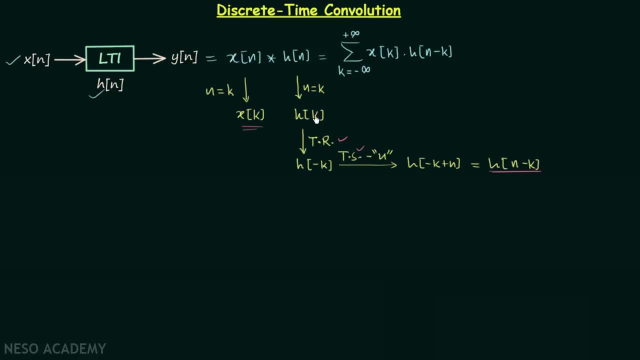 reversal and time shifting operations on hk. So the only thing required is to multiply this signal and this signal and then perform the summation. So this is what we do in convolution operation when we are dealing with discrete time LTI system and the discrete time signals. Now let's move on to our 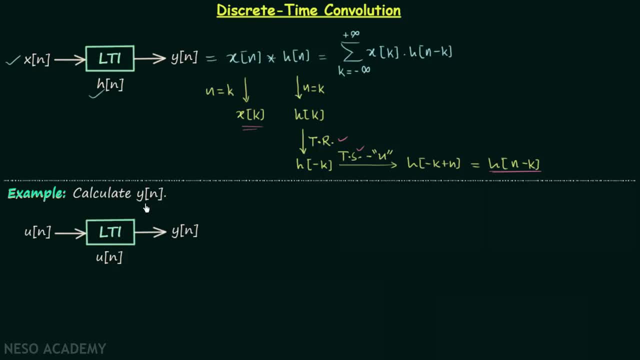 example in which we will calculate the output yn of an LTI system having input, having input as un and having the impulse response as un. So the input and impulse response, both are unit step sequence. therefore, output yn will be equal to the convolution of un with un. 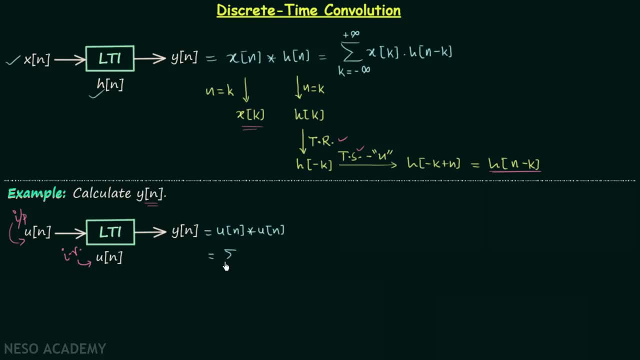 And the convolution is equal to summation k, equal to minus infinity to plus infinity, uk multiplied with un minus k. So, keeping all these processes in mind, let's begin our solution. We know we are having unit step sequence as the input, the LTI system, and we are having unit step sequence as the impulse response of 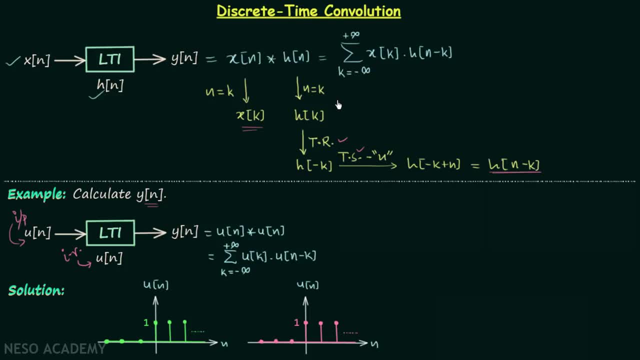 the LTI system, and from here we can see that we are replacing variable n by a dummy variable k, and both n and k are integers. so let's quickly replace variable n by variable k. this will give us signal uk as the input signal, and the impulse response will now become uk as well. and you can notice one thing: that 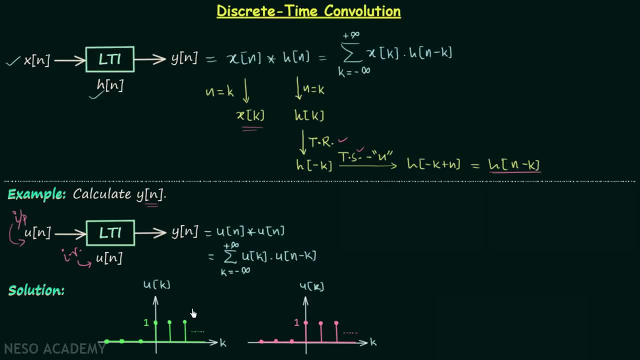 by replacing variable n by k. there is no effect on the plot of the signal. and now we will leave the input signal as it is and we will perform the time reversal operation on the LTI system impulse response. so we will leave the input signal as it is and we will perform the 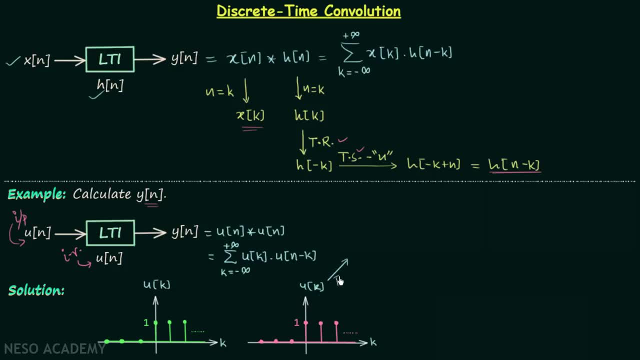 time reversal operation on the impulse response. and we know, in case of time reversal operation we simply flip the signal waveform about the y-axis. so flip the signal waveform about the y-axis and you will have the plot like this. so this is the plot of the LTI system. 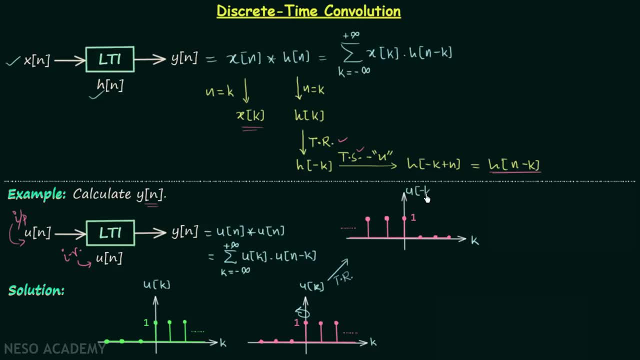 so this is the plot of signal he minus k, and therefore we have a new signal after performing the time rehearsal operation and upon this new signal will perform the time shifting operation by n. so let's perform the next operation, that is, the time shifting operation by integer. 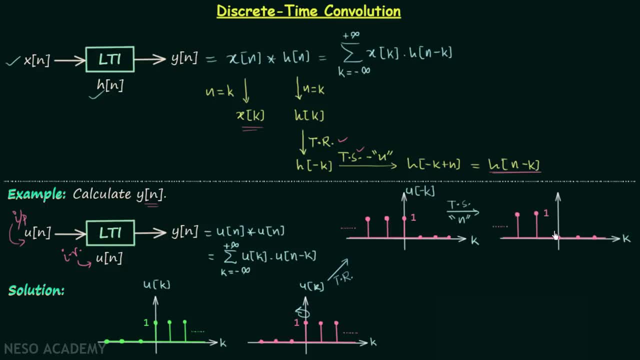 and we will have the waveform like this. you can see that the waveform almost is shifted towards the left by n and this is the signal: u n minus k. So we have u n minus k and we have u k. Now let's analyze what will happen when we multiply u k and u n minus k. 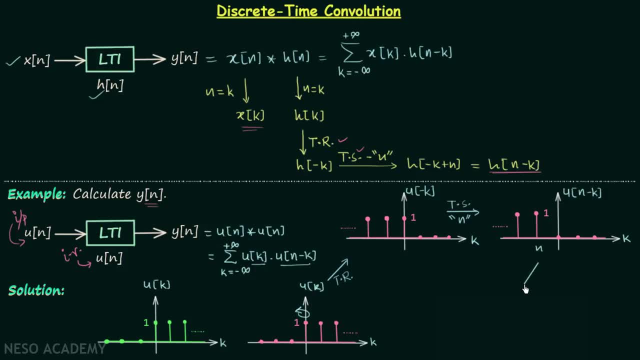 depending on the value of n. So here is the plot in which I have included u n minus k. You can see the pink plot representing u n minus k and I have included u k. The green plot is representing u k. Now let's say n is equal to minus 1.. This means n is less than 0.. Now, when n is less than 0,, 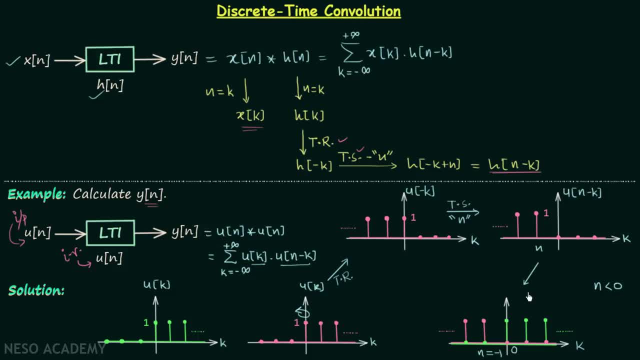 it is equal to minus 1.. You can see that the result of multiplication is equal to 0 for all the values of k. For example, when k is equal to 0, you can see that the green plot is having the value equal to 1.. This means u k is equal to 1, but the pink plot is 0. This means u? n minus k. 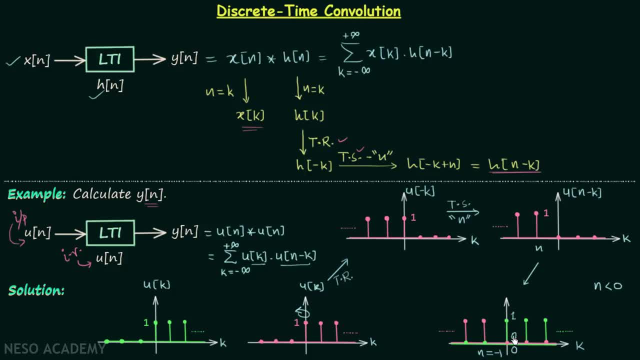 is equal to 0. So 1 multiplied to 0 will give you 0.. Similarly, for all the values of k, we are going to get 0 when n is less than 0. And we are performing the summation from k equal to minus infinity to plus infinity. 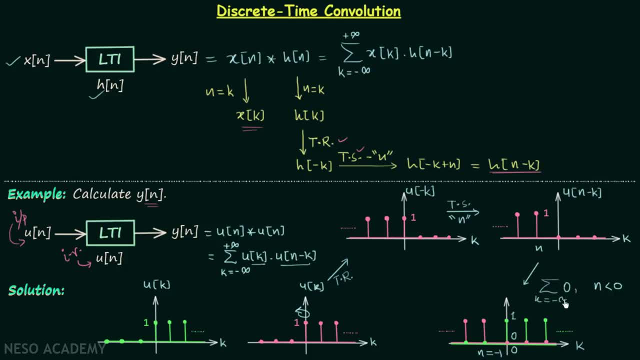 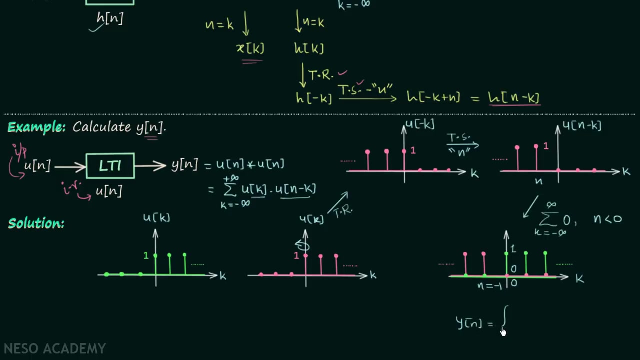 So we have summation k equal to minus infinity to plus infinity And as we are having zeros for all the values of k, if you add zeros from minus infinity to plus infinity, we are going to get 0. Therefore, the output y- n is equal to 0 when n is less than 0.. 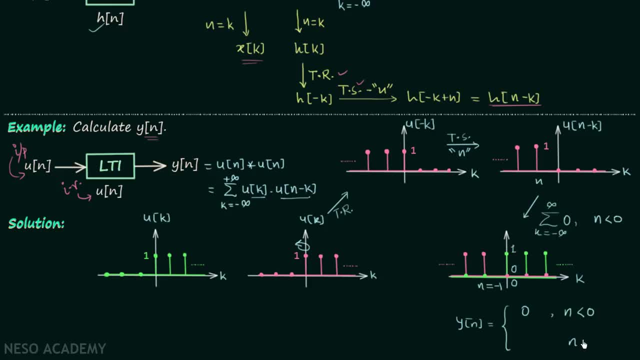 Now we will consider the next possibility, and this time n is greater than or equal to 0.. When n is greater than or equal to 0, let's take one example of this: u n minus k is equal to n is equal to plus 2.. The plot: 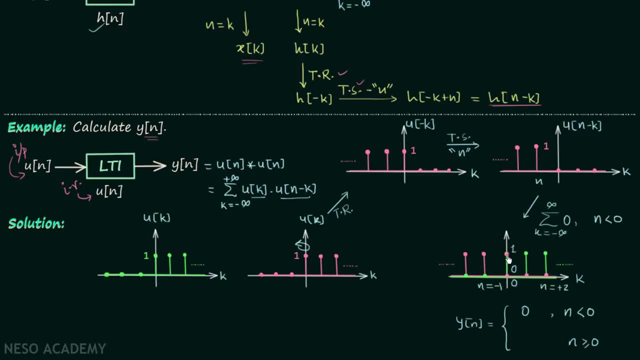 of u n minus k will now shift like this: Initially you can see that when n is less than 0, when k is equal to 0,, u n minus k was zero, but now it is 1.. Similarly, when k is equal to 1,. u n minus k is now 1.. k is equal to 0, u n minus k is now 1.. Now, in order to interestingly evaluate these two 403 values here, glue and the Googling property is supposed come to. 玩 ourractor for food героism. So whenever we solve a puzzle or 18 clears, can we Hop EN Dougl program and fill out the value of log Nemos? you should learn different terms in this course and stress function. So in order to solve, Solve All Problems, inrecipid curve types. 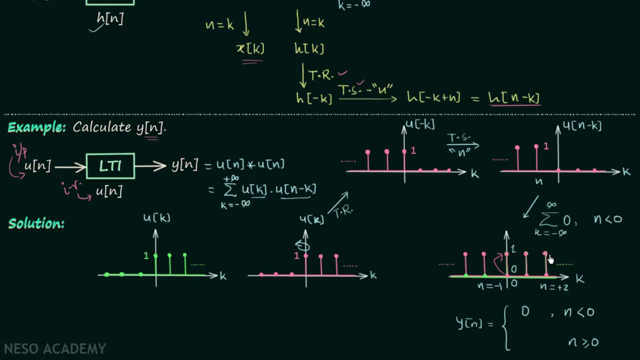 let's leave radian and solve the problem in message query. The deeds of Solve All Problems in to 2, un-k is now 1 and for the other values of k which are greater than 2, un-k is still 0.. 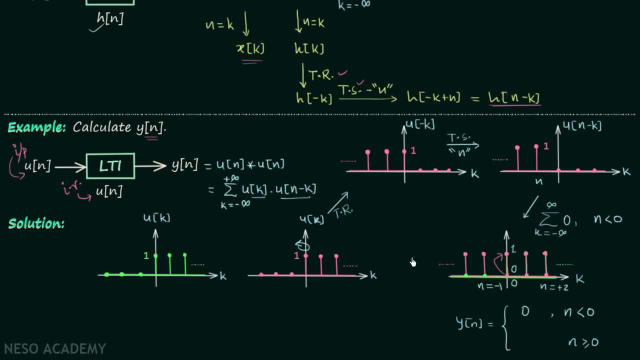 Now let's calculate uk multiplied to un-k for the different values of k, And we will first consider the case in which k is negative. This means k is less than 0. For example, when k is minus 2, you can see that un-k is equal to 1, but uk is equal to. 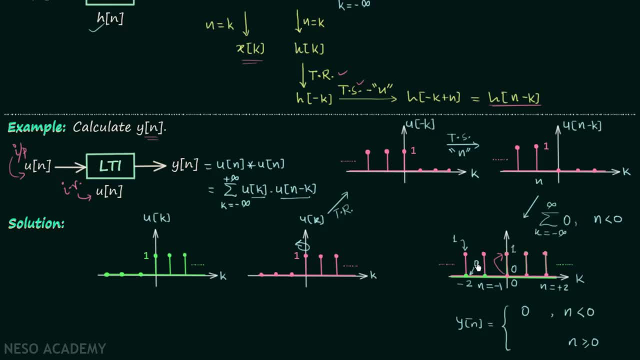 0.. So 1 multiplied to 0 will give you 0. So for all the values of k which are negative, we are going to get the product equal to 0. And as we are performing the summation, we will add all the 0s, starting from k equal. 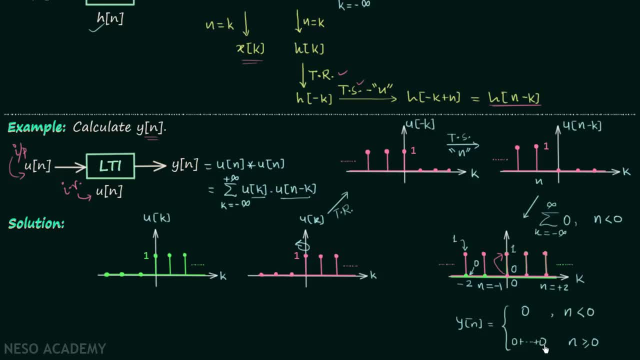 to minus infinity. After this, when k is equal to 0, you can see that un-k is equal to 1 and uk is also equal to 1.. So 1 multiplied to 1 will give you 1.. So we will add 1.. 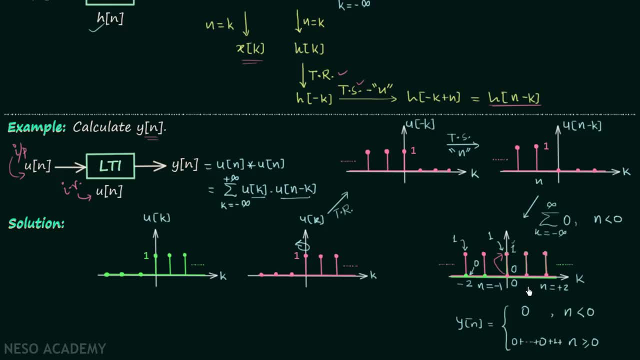 Similarly, when k is equal to 1,, again we have uk and un-k equal to 1.. So the product is 1.. So we will add 1.. Similarly, when k is equal to 2, we have 1 more 1.. 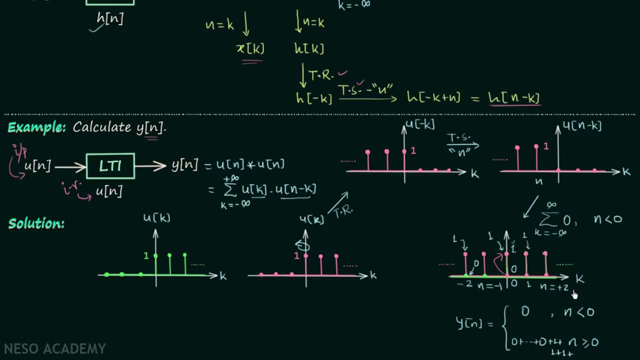 And after that, when k is equal to 3, uk is 1, but un-k is now 0. And it will remain 0 up to k, equal to plus infinity. So again we have so many 0s, followed by 1.. 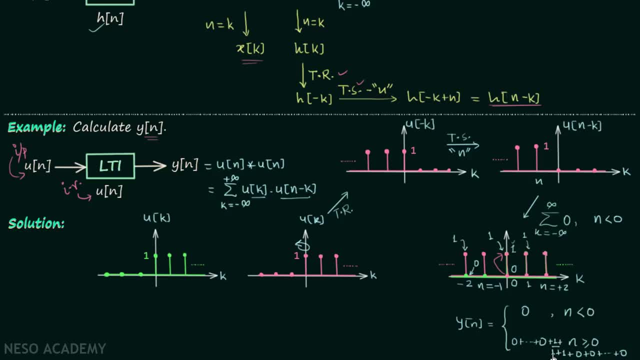 Now, when you add them up, you will get 3.. 1 plus 1 plus 1.. We will give you 3.. So I will write down 3 as the output yn when n is equal to 2.. So we are having 3 when n is equal to 2.. 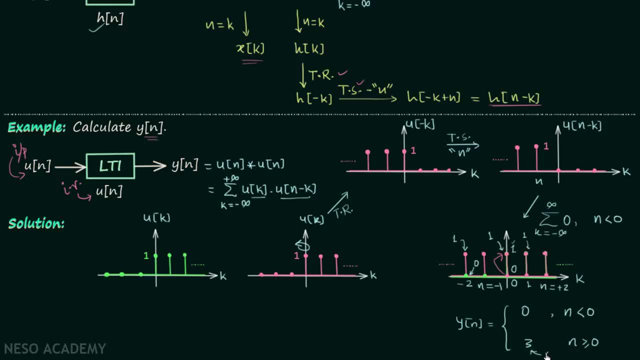 And from here we can say that yn is equal to n plus 1, because n is 2 and we are getting 3.. So 2 plus 1 is 3.. We will find out the general answer after understanding the fact that it is going to. 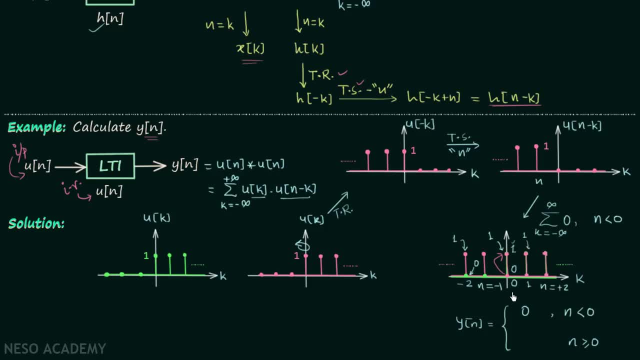 be 1.. Now we will add the sum that it is good to perform this summation from zero to n, because from 0 to n we are getting the result of multiplication equal to 1 when n is greater than or equal to 0.. 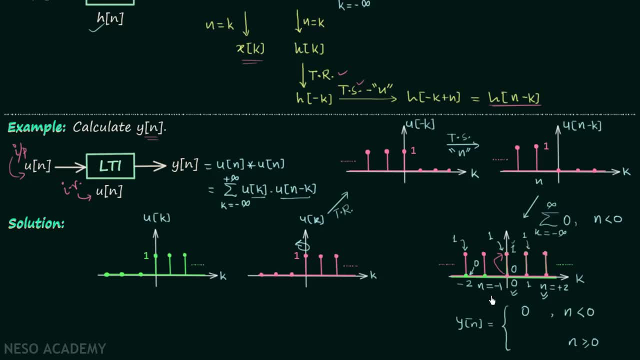 And all the other values of k which are outside 0 to n are giving us the result of multiplication equal to 0. So we will perform the summation from k equal to 0 to k equal to n- n, and the summation we will perform is of 1.. Let's understand how we are getting n plus. 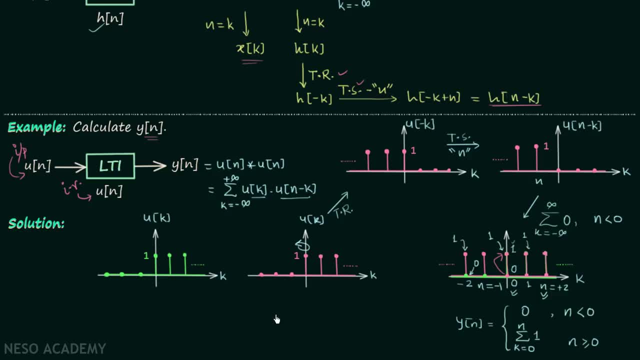 1. when we perform this summation, We are starting from k equal to 0. We are having 1 when k is equal to 0. Then we have 1 again when k is equal to 1, and we will have 1 all the way. 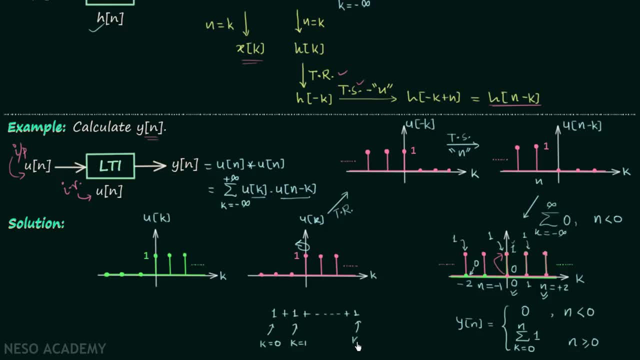 to k equal to n. Now, if we consider this portion of the summation from k equal to 1 to k equal to n, we are adding 1's n times. Therefore we can write 1 multiplied to n. and if we consider: 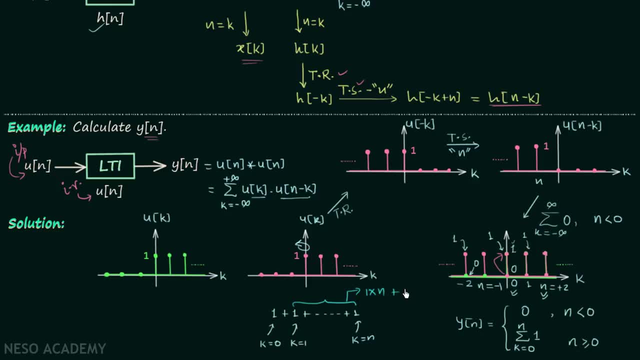 this one present at k equal to 0, we will add one more, 1.. So from here we are getting n plus 1.. so in place of summation k equal to 0 to n 1, we can write: we can write n plus 1. 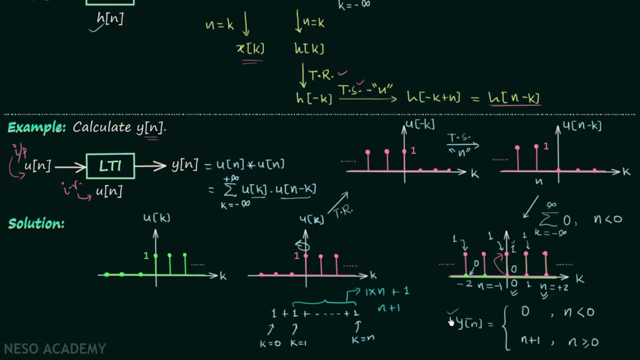 so this is how the output yn of the LTI system is defined, and we know the unit step sequence: un is equal to 0 when n is less than 0 and it is equal to 1 when n is greater than or equal to 0. now let's multiply. let's multiply n plus 1 to un. when you multiply n.